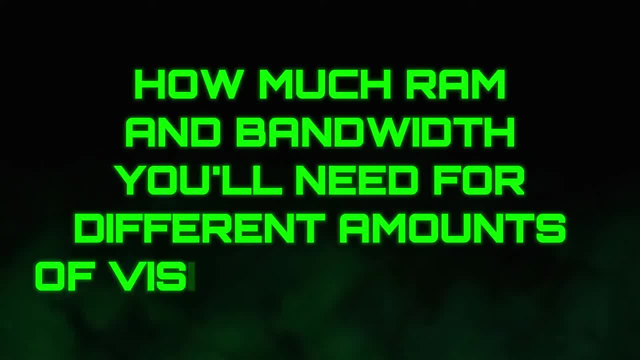 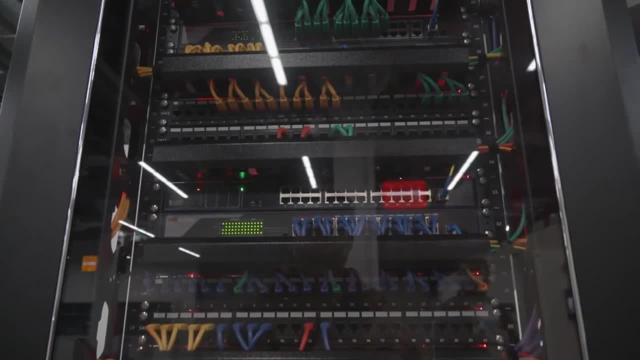 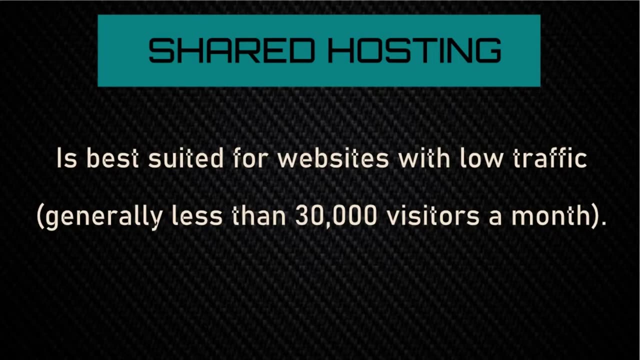 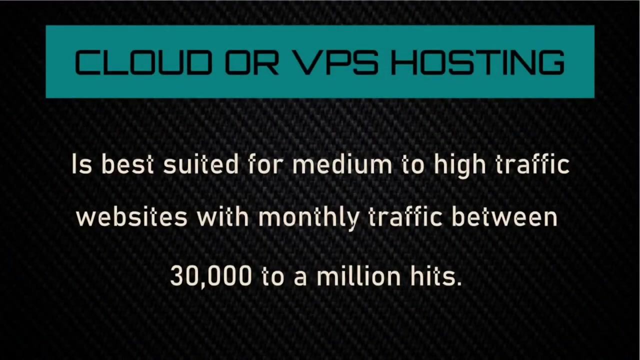 How much RAM and bandwidth you'll need for different amounts of visitors per month. A web server with adequate resources ensures excellent performance and user experience. Shared hosting is best suited for websites with low traffic, generally less than 30,000 visitors a month. Cloud hosting or VPS hosting is best suited for medium to high traffic websites with. 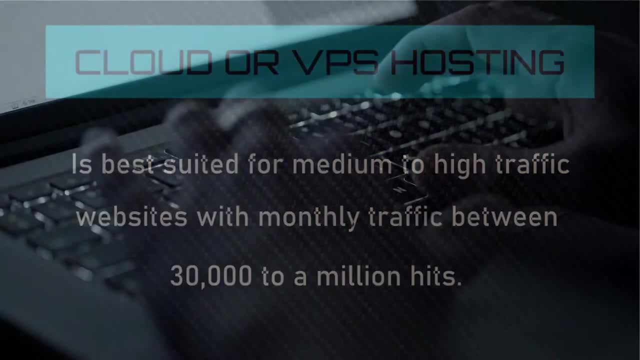 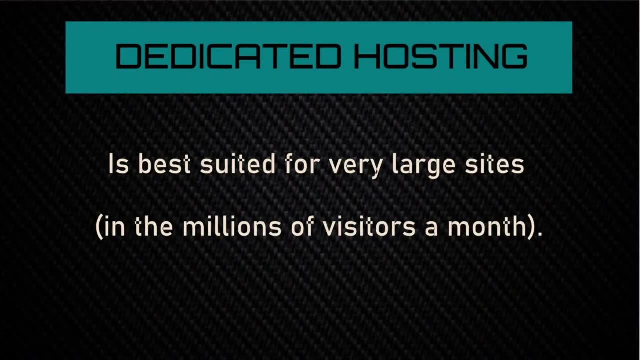 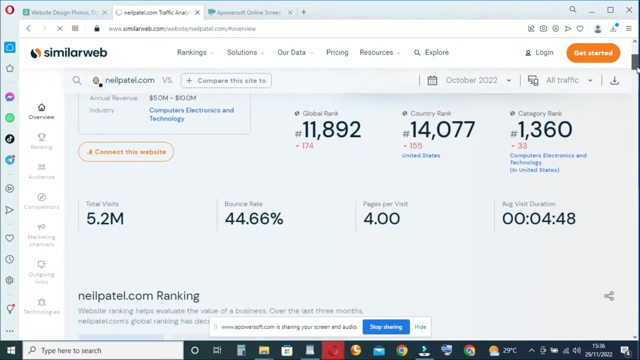 monthly traffic between 30,000 to a million. Dedicated VPS hosting is best suited for very large sites in the millions of visitors per month. Every plan has a limit of live users or concurrent visitors. it can accommodate on your site Concurrent users or number of page requests per. 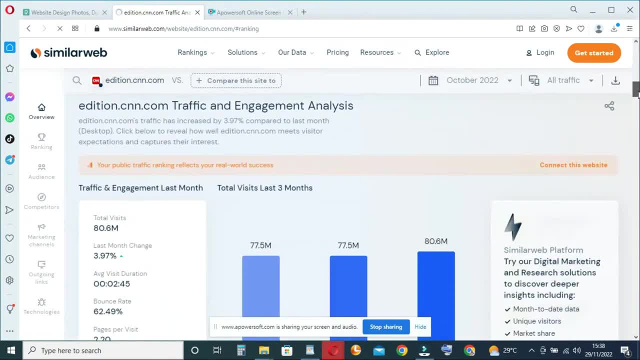 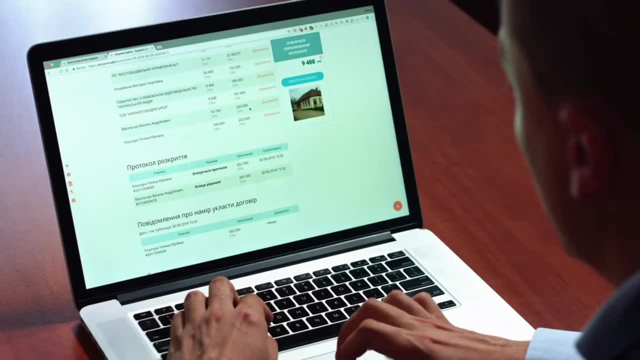 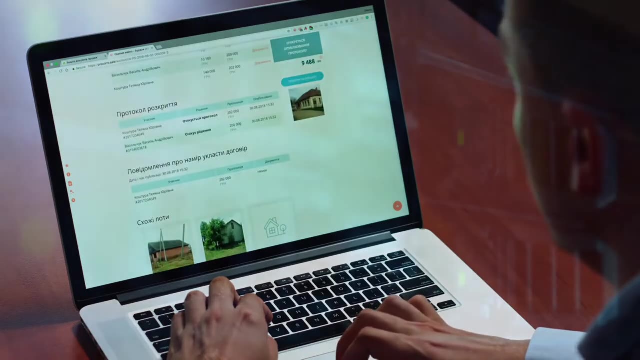 second is a standard way of effectively planning, measuring and managing hosting capacity. Whenever you reach a real-time concurrent visitor limit for your hosting plan, the CPU usage will reach 100% and your site will start loading very sluggishly and eventually end up in a 504. gateway error message to your potential visitors. How much traffic different hosting resources can handle. Please note that these numbers are just estimates. They are not set in stone, because there are a lot of variables that can cause these numbers to differ from website to website. A 1GB RAM cloud hosting plan can accommodate up to 75 concurrent visitors. 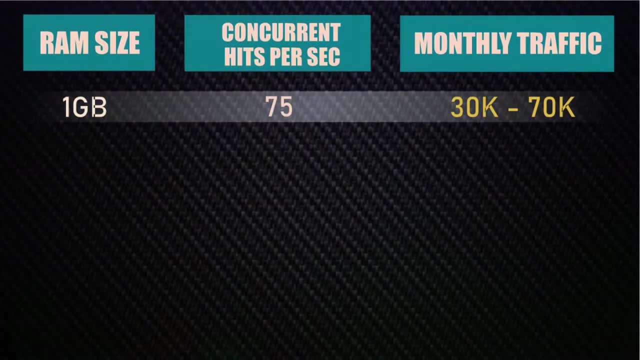 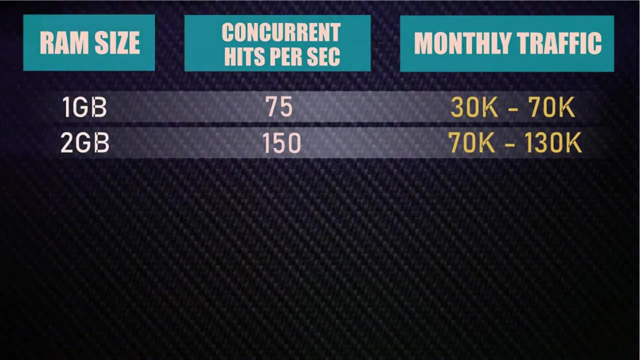 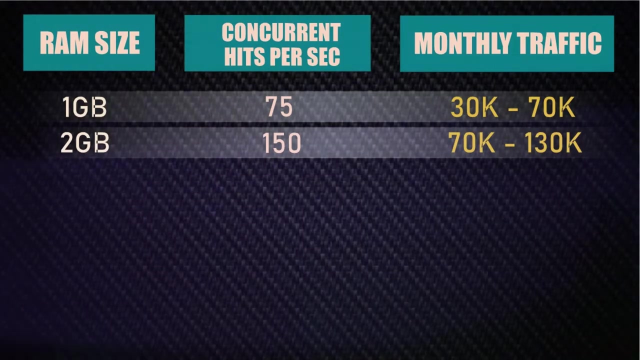 or real-time hits per second and deliver up to 30,000 to 70,000 monthly traffic. A 2GB RAM cloud hosting package can accommodate up to 150 concurrent visitors or real-time hits and deliver up to 70,000 to 130,000 monthly visits. A 4GB RAM cloud hosting package can accommodate up to 150 concurrent visitors or real-time hits and deliver up to 70,000 to 130,000 monthly visits. 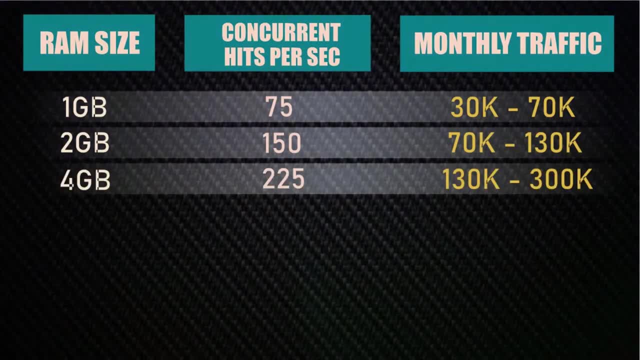 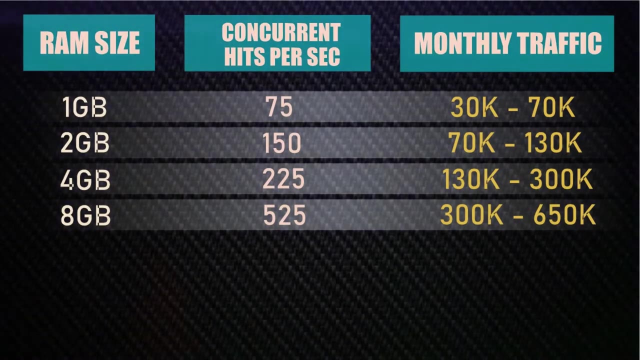 A 4GB RAM cloud hosting package can accommodate up to 225 concurrent visitors or real-time hits and deliver up to 130,000 to 300,000 monthly traffic. An 8GB RAM cloud hosting plan can accommodate up to 525 concurrent visitors or real-time hits and deliver up to 300,000 to 650,000 monthly traffic. 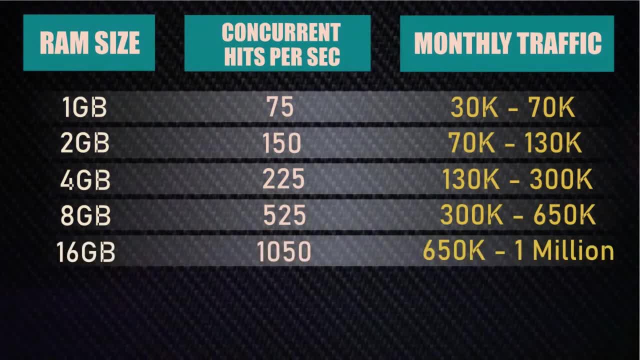 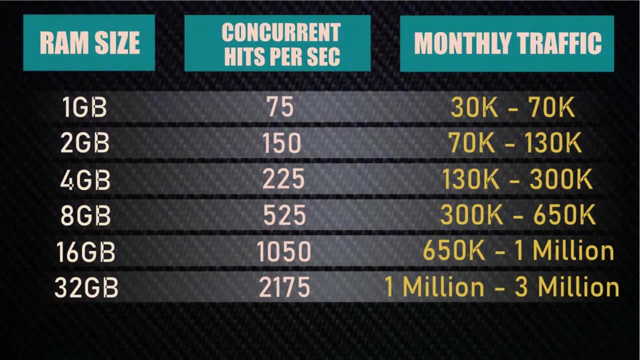 A 16GB RAM cloud hosting package can accommodate up to 1,050 concurrent visitors and deliver up to 650,000 to 1,000,000 monthly visits. A 32GB RAM cloud hosting package can accommodate up to 2,175 concurrent visitors or real-time hits and deliver up to 1,000,000 to 3,000,000 monthly traffic.